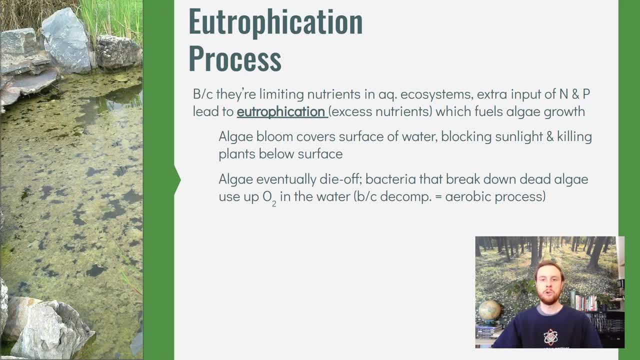 water start to break them down Now, because decomposition in the water here is an aerobic process. the bacteria are going to use up a lot of oxygen, So they're going to decrease the dissolved oxygen level in the water as they use it up to break down the dead algae as well as. 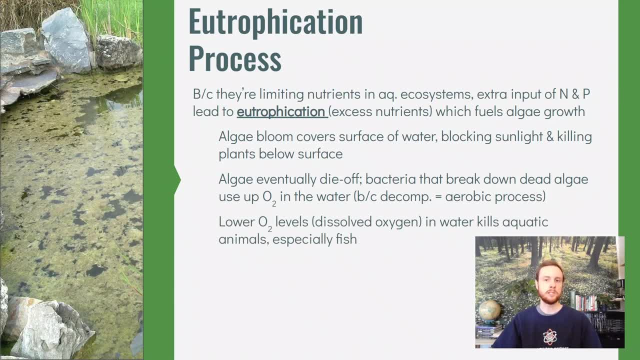 the other dead plants beneath the surface. Basically, what this does is lowers dissolved oxygen, So it just continues to go lower and lower. That results in more and more aquatic species dying, because they need that dissolved oxygen for respiration- Fish especially because 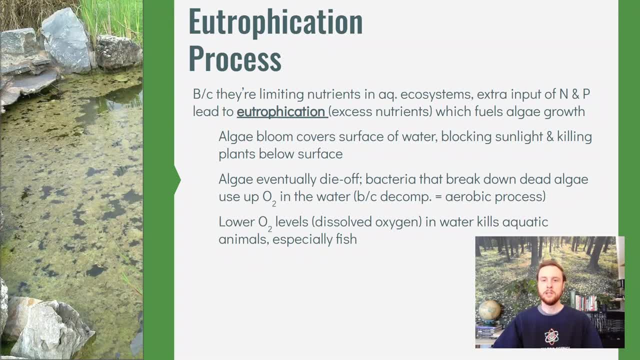 they're larger organisms, they're going to demand a little bit more oxygen. We'll take a look at this later in the video. The step is just continuing here again, where bacteria are again using up even more oxygen to break down more dead aquatic organisms, And what we get pretty quickly is a. 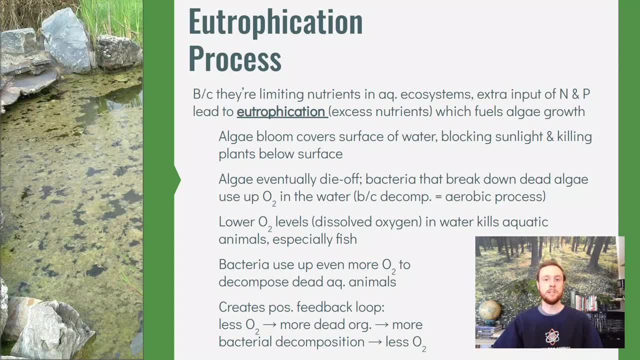 positive feedback loop. Remember that a positive feedback loop does not mean it's good. In this case it's bad, or at least it's bad from the standpoint of dissolved oxygen. So we're going to look at a positive feedback loop. It's driving the conditions of the water away from a stable 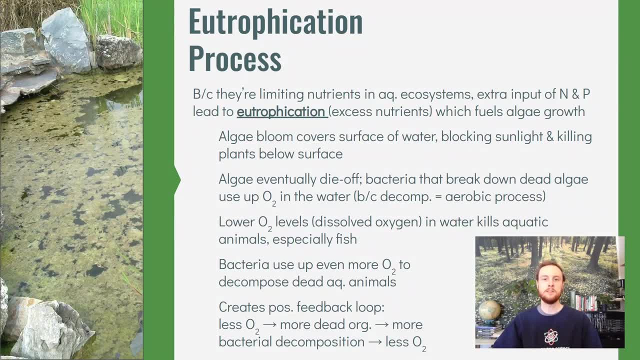 state, And so positive feedback loop just refers to the fact that the input, in this case fertilizer or nitrogen or phosphorus, is amplifying the effect, And so there's less and less oxygen, resulting in more dead organisms, which results in even less oxygen as bacteria break down those. 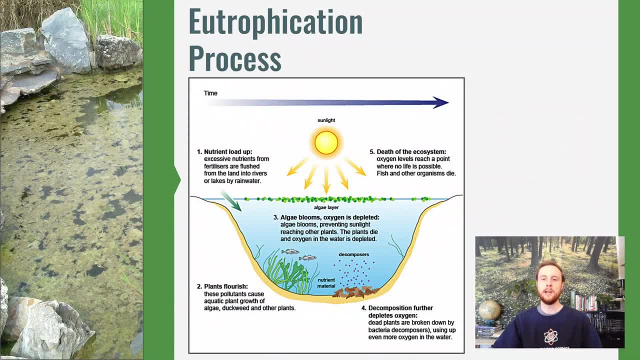 dead bodies. Here's a really helpful diagram that will help you walk through the steps here. help suggest that you draw this diagram in your notes, that you write these steps down. It really just reiterates everything that I just explained with the bullet points, But it's so helpful to have this. 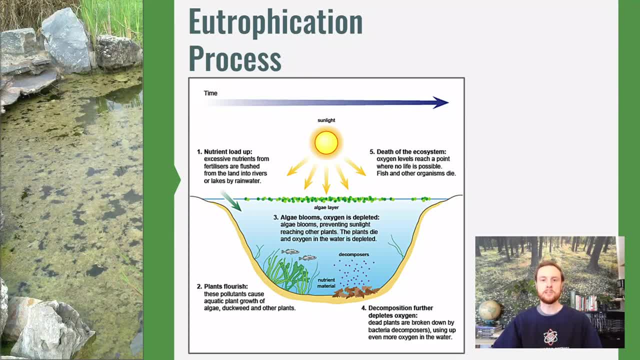 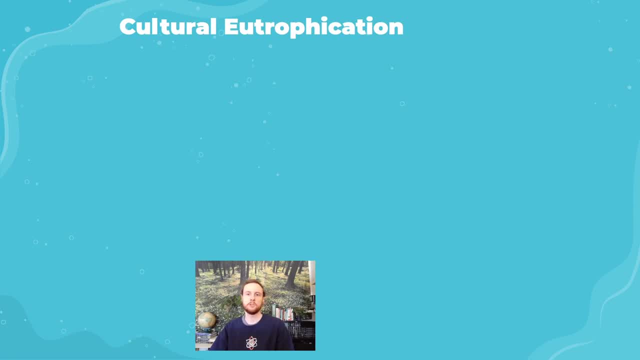 visual, And so, again, highly recommend that you sketch this out and write out some of these steps. So now we'll talk specifically about cultural eutrophication. The word cultural, here in front of eutrophication, just means that this is anthropogenic or human driven nutrient pollution. 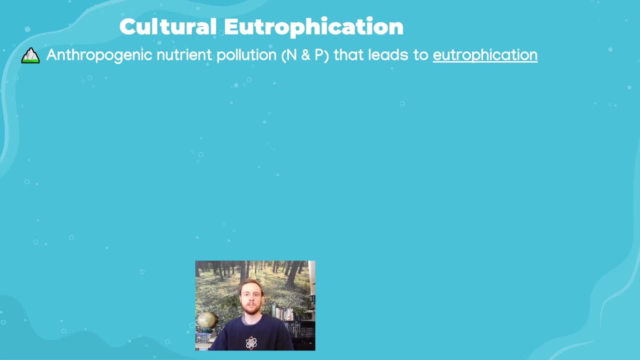 that's causing the eutrophication. This is important to point out, because eutrophication is not a process that's limited to human pollutants. It can also just be something that naturally occurs in ecosystems- aquatic ecosystems, that is, over time, And so on the next slide, we'll actually 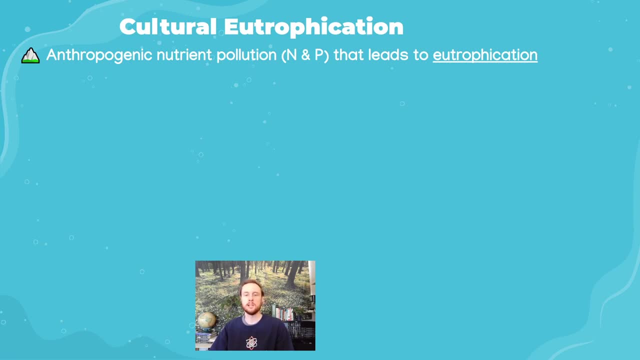 look at how bodies of water can be naturally eutrophic, And so it's not something that's only caused by humans, And so you want to be aware of this, because you may see the word cultural in front of eutrophication on an exam. So it's important not to freak out and not to think this is something. 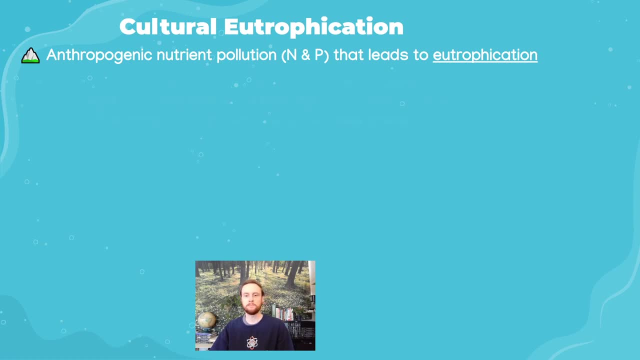 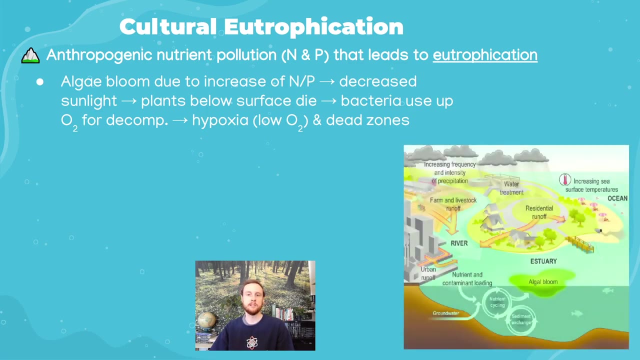 different that you don't know. It just means specifically human caused. So let's take a look at the steps one more time Very quickly. we just want to remember that the algae bloom is key, So we have that here in this diagram. That's going to block the sunlight. And then when algae and other plants beneath the 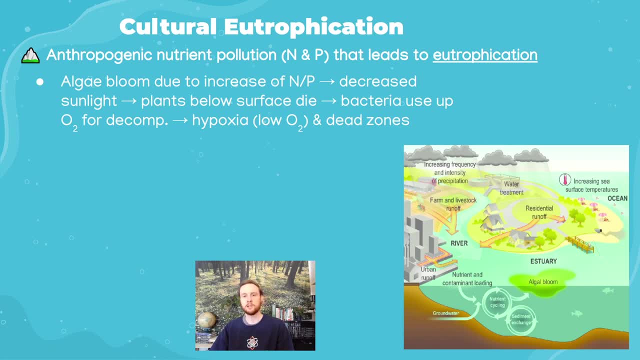 surface die. decomposers break down their bodies, ease up the oxygen and now the water is hypoxic, or has undergone hypoxia, which is having a incredibly low oxygen level, to the point that we can't really support life. We call that a dead zone. So what are the sources of the nutrients? 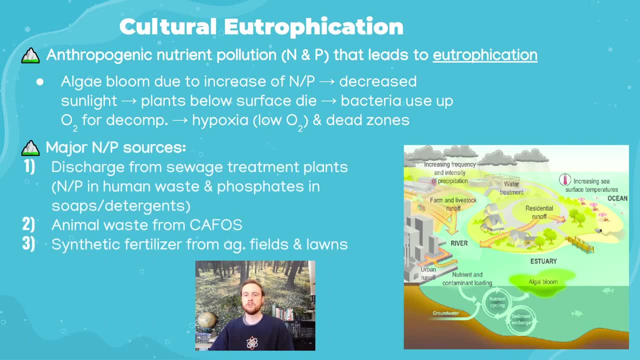 that can cause eutrophication. Well, take a look at the slide, At some of the key sources here. the first one is going to be the discharge from wastewater treatment plants. So in this diagram here, there's a red circle around the wastewater treatment plant. Now 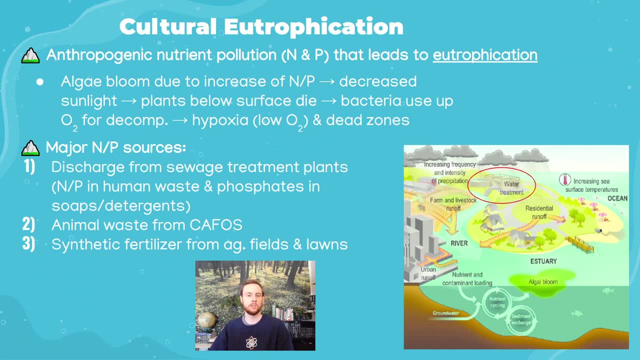 while these facilities are designed to specifically remove nutrients and other pollutants from human wastewater, that doesn't mean that they always are able to bring those levels completely down to zero. Another example of how nutrients could be added to a body of water from the discharge of a water. 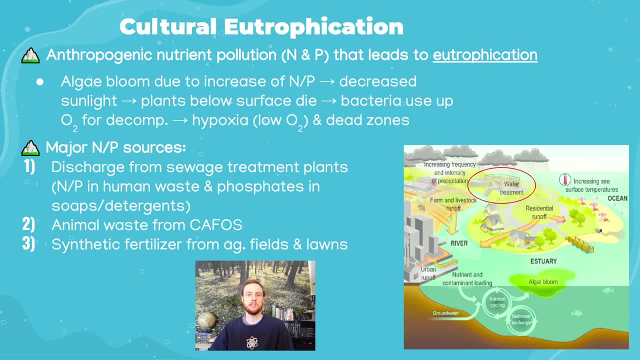 treatment plant is if there's a really heavy rain event. So sometimes cities will have a lot of rain. Sometimes cities will have a combined stormwater runoff and sewage treatment system together, And if it rains really hard these facilities can actually flood and then they're discharging raw sewage directly into a body of water. 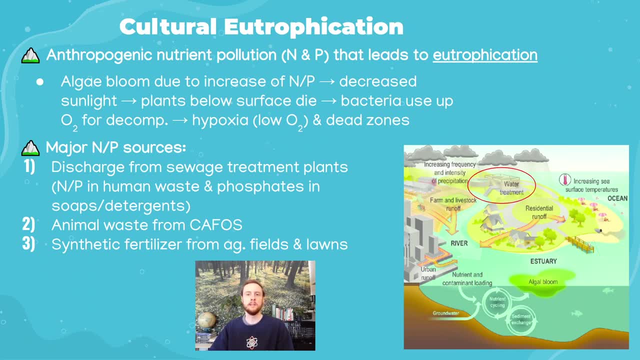 So remember that human waste, just like animal waste, will contain ammonia, So that's a source of nitrogen. It's also going to contain phosphorus, And then even just the detergents we use or the soaps that we use, those go down our drains. 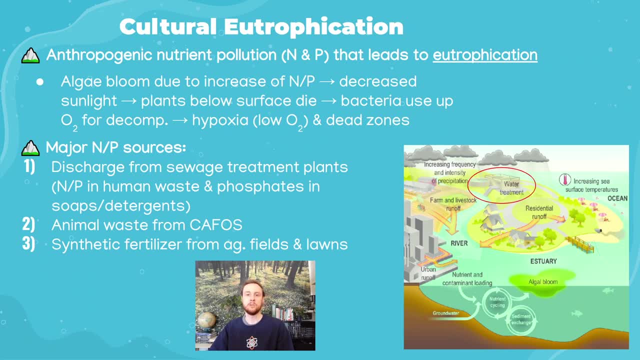 They go to our water treatment plants And if those processes don't completely remove the phosphates, then they're going to go down our drains. And if those processes don't completely remove the phosphates, then those phosphates in the detergents can also contribute to eutrophication. 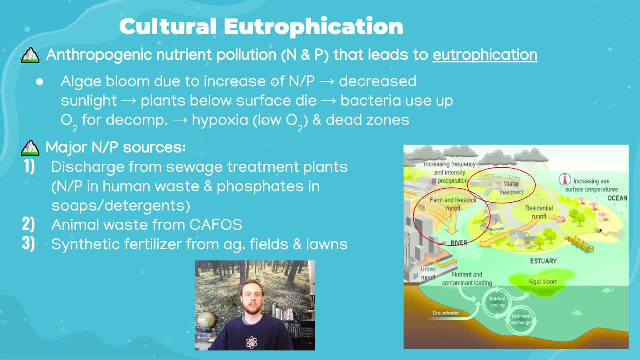 Then we have agriculture, And so remember that CAFOs, or concentrated animal feeding operations- feedlots, you might know them, as they're going to have a lot of animal waste stored at them, And so these are typically in manure lagoons. 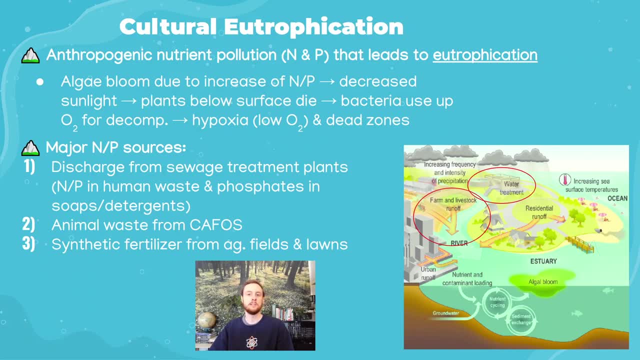 But if best management practices aren't followed, those can easily flood or they can leach into the groundwater and that can infiltrate into these rivers, And there we have again the ammonia from these animals' waste from their eutrophication, And so that's a source of nitrogen. 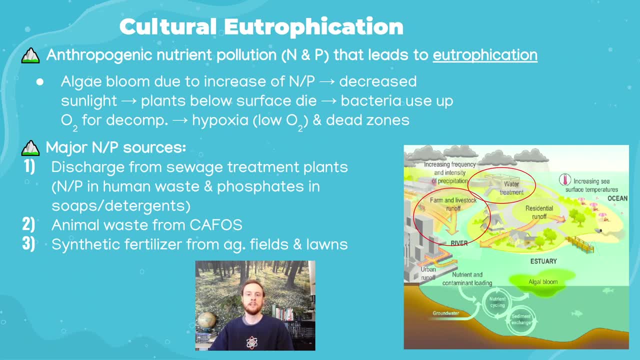 And then if there's a lot of nitrogen in the water treatment plant, then that's a source of nitrogen. And then if there's a lot of nitrogen in the water treatment plant, then that's a source of nitrogen. So those can be sources of nutrient pollution as well. 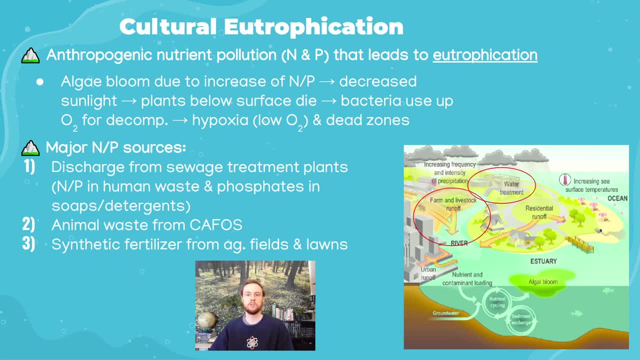 And then just agricultural fields or crops can also contribute to this, as farmers are applying synthetic fertilizers which have a lot of nitrate, And when it rains, those nitrates- or the phosphates in some cases- are going to be washed into the surrounding tributaries that are around the farm. 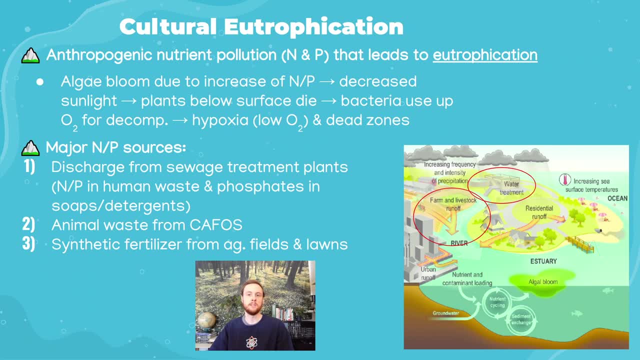 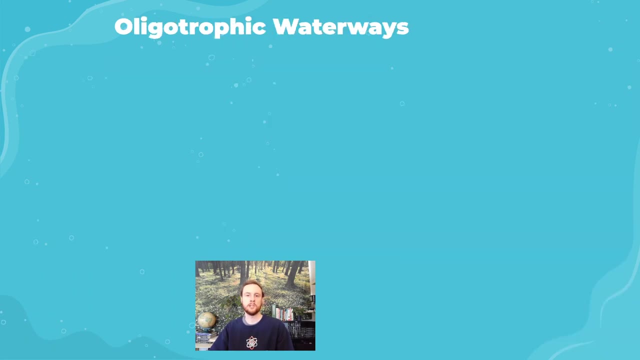 And that's going to eventually empty into this river, And there we have numerous ways that phosphates and nitrates are entering rivers and streams. Remember, major ways here that humans contribute to this are wastewater treatment plants and agriculture. So, as I mentioned earlier, eutrophication is not limited to human causes. 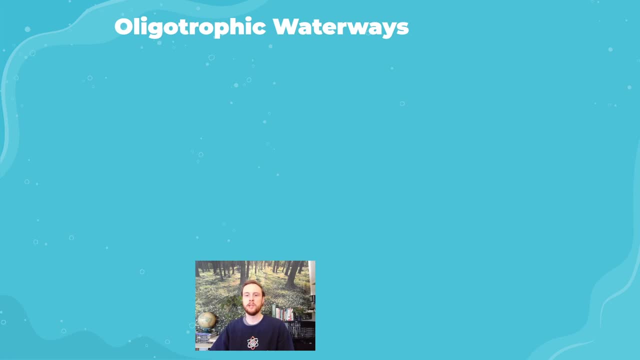 Waterways can be naturally eutrophic, And before we look at that, though, we have to understand what an oligotrophic waterway is. So an oligotrophic waterway is one that has low nutrient levels, stable algae populations and high dissolved oxygen. 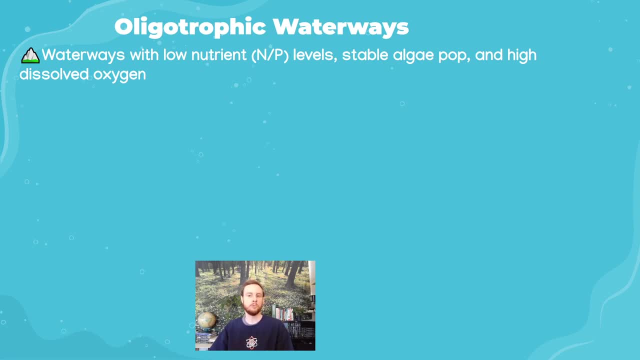 Now think about what happens with eutrophication. Because of the lower nutrient levels in oligotrophic waterways, they're not going to have these huge algae blooms, They're not going to have a ton of plant death due to the sun being blocked. 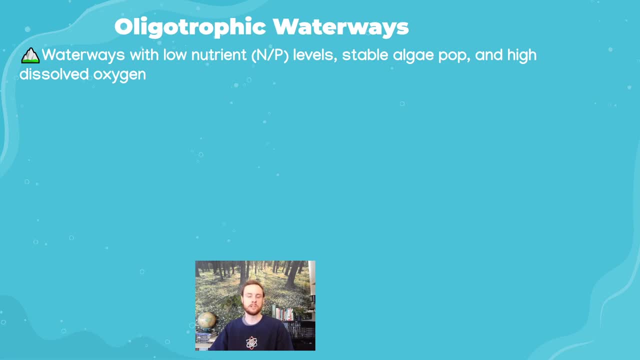 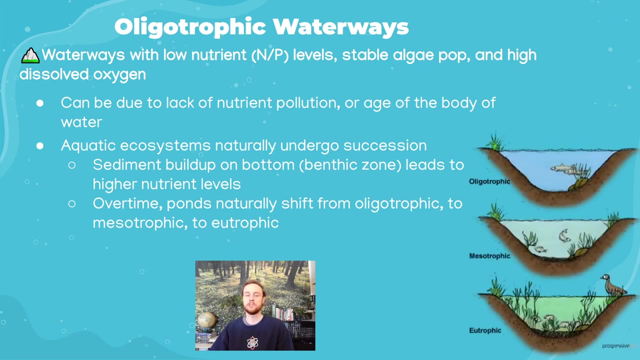 And so they're not going to have a ton of microbes using up their dissolved oxygen. This could be due to lack of nutrient pollution, but it can also just be due to the age of the body of water. So ponds, especially, are a great example of how succession actually occurs in aquatic ecosystems, just like it does in terrestrial ones. So ponds, especially, are a great example of how succession actually occurs in aquatic ecosystems, just like it does in terrestrial ones. And so if we look here, as the time goes on that a body of water has been in existence, it's going to gradually fill in with sediment along the bottom. 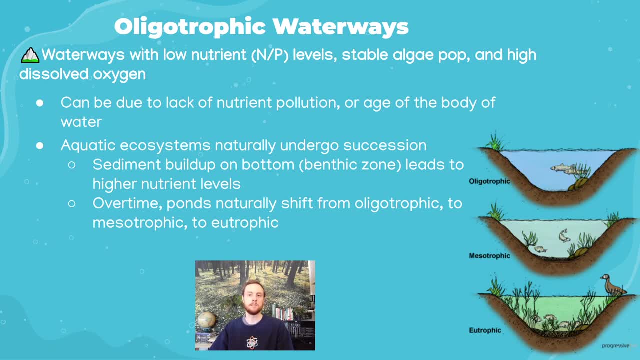 And so, if we look here, as the time goes on, that a body of water has been in existence, it's going to gradually fill in with sediment along the bottom. Now this could be from runoff adding the sediments in. It could be just from the plants and organisms dying, being decomposed, broken down and added to the sediment layers. 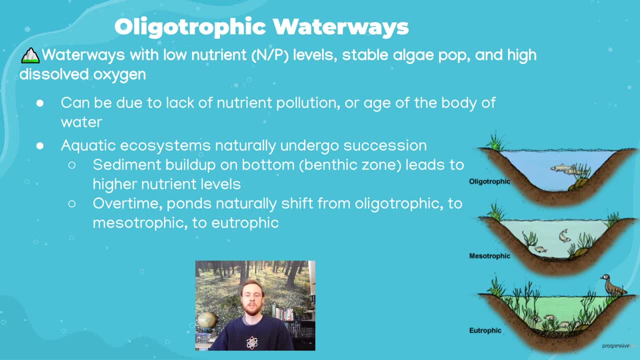 But basically the bottom of the body of water, or the benthic zone, is going to become deeper and deeper. It's going to have more and more sediments. Those sediments have nutrients that they release into the water. with time, a waterway will naturally just start to become eutrophic. This is primarily limited to 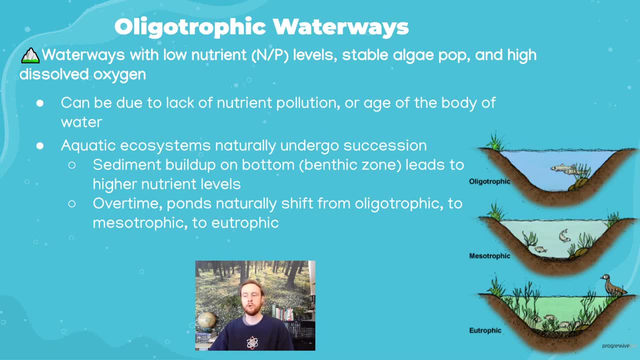 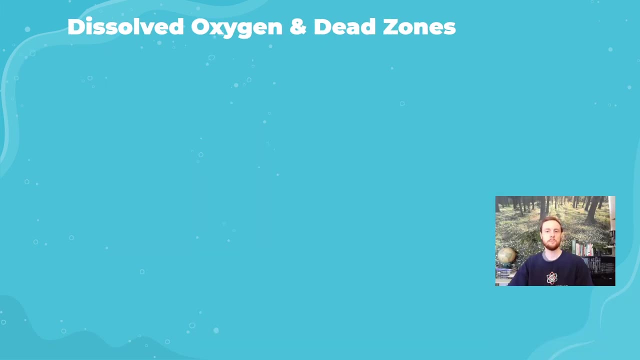 ponds and lakes, because rivers and streams have the flow of water which can alter the way that sediment builds up on their bottoms. But essentially again, eutrophic waterways are not just limited to human pollutants. it can happen as a result of natural aquatic succession. So we'll wrap up today. 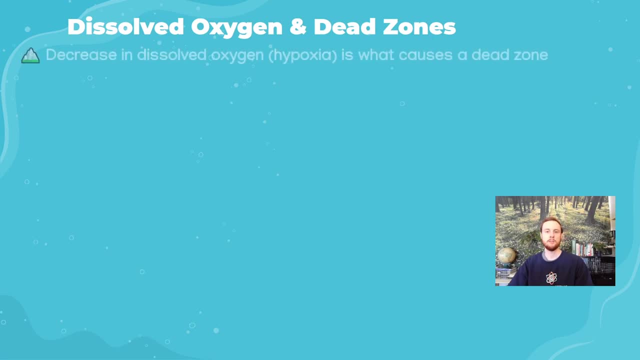 by talking about dissolved oxygen and dead zones. So a reminder that the actual cause of the dead zone is hypoxia or low oxygen conditions. Another instance of a word here where root terms are helpful. so hypo is low or too little and ox refers to oxygen and the suffix ia refers to kind of a. 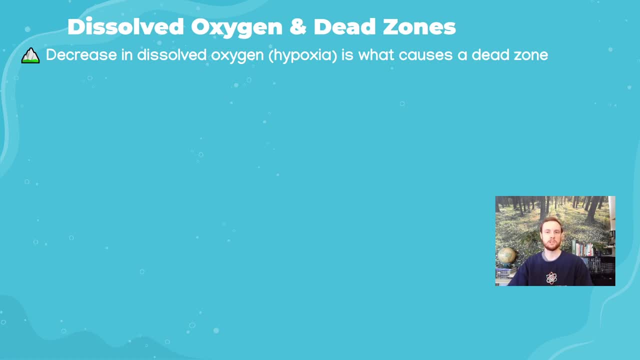 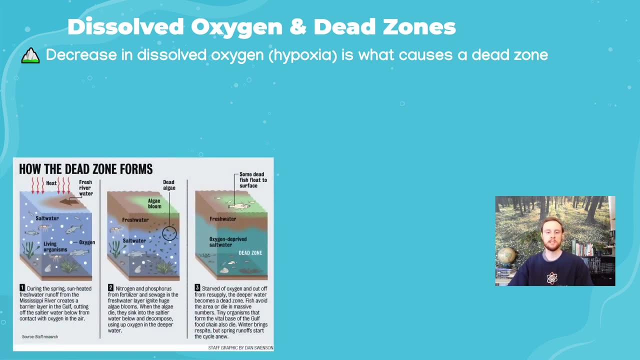 condition or a state of being. So it's the state of being in a low oxygen condition, And so we can look at a helpful diagram here, and we're going to kind of use the Gulf of Mexico as a case study here. And so what happens is in the left hand side of this diagram, panel one we're going to 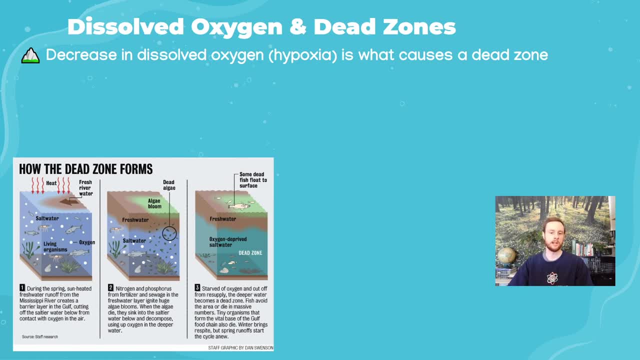 have a thriving aquatic ecosystem where there's a lot of dissolved oxygen. You can see the white little circles there represent that. we have tons of organisms in the Gulf. But then we have fresh water that's starting to come in and heat, which is also an important part of the equation. So 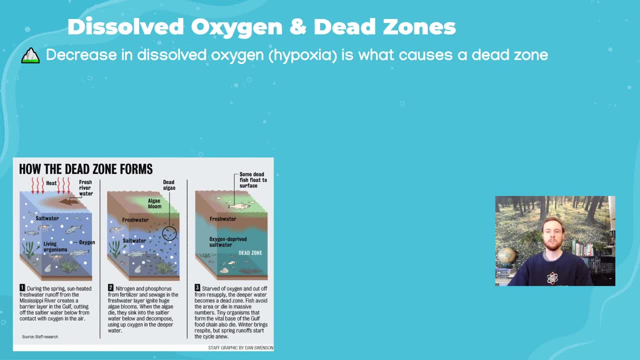 as temperature rises, especially in the summer, that's going to lead to algae blooms, because those conditions are more favorable to the algae. They reproduce at a faster rate as the water warms up. So then when we look in the center in panel two now we have an algae bloom. So the sunlight 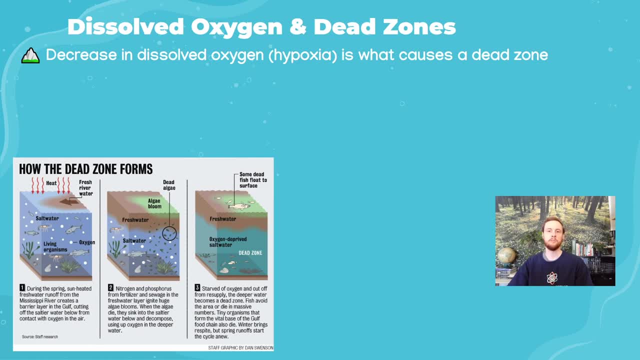 is being blocked by this thick, you know, clump of algae on the surface. The algae themselves are starting to die. Some of the aquatic plants are starting to die beneath the surface. That's going to lead to all of these microbes or bacteria breaking them down and using up oxygen. Now on, 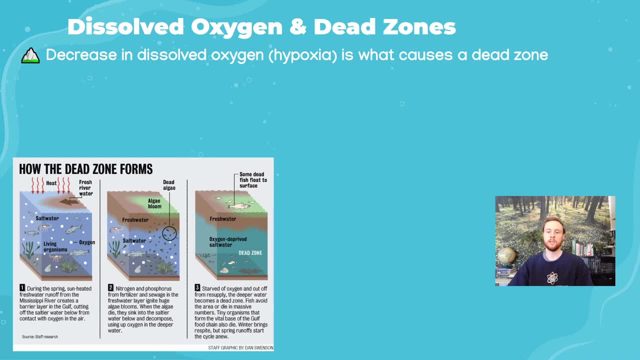 the third panel, we have basically a dead zone. We have so little dissolved oxygen that really no aquatic life can be supported, And so we have fish that are floating up to the top because they've died. We have plants and other crustaceans or other organisms on the bottom that have died. 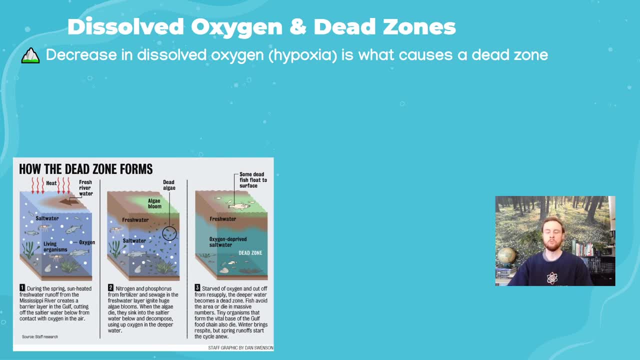 And so we need to think about here: why does this actually happen? Why does a decrease in dissolved oxygen lead to all of these organisms dying? Well, it's important to remember that, just like terrestrial life, so just like organisms on land, aquatic organisms need oxygen to survive. They're 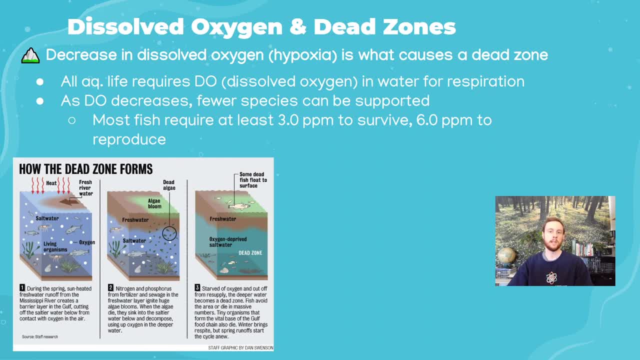 going to undergo cellular respiration, just like, you know, animals on land, or just like plants on land, And so, without it, they're not going to be able to respire and they're not going to be able to produce energy, and they're going to die. Now we'll take a little bit closer look at 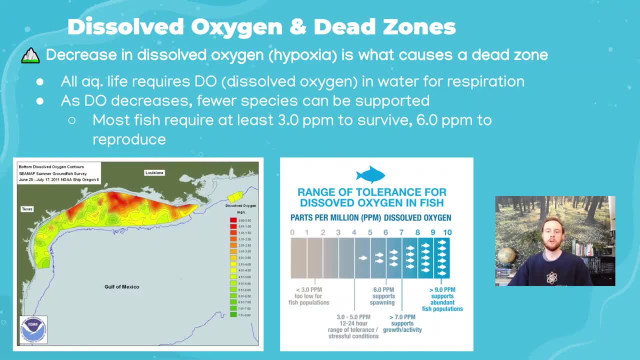 fish as kind of a model organism here, And fish are a great example of how range of tolerance comes into play here as well. So most fish can survive for a short period of time in waters that are three to five parts per million dissolved oxygen, And so I want to point that out there. the PPM. 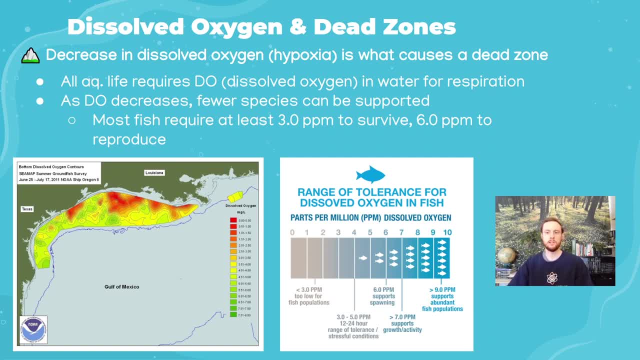 stands for parts per million. That's how we measure dissolved oxygen in a body of water. But when we get up to six, that's kind of the minimum threshold for most fish populations to actually reproduce and actually sustain a stable population. So if we look at this map from NOAA from the summer, 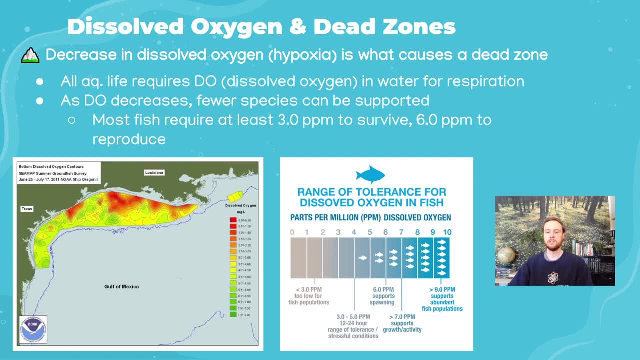 of 2011 in the Gulf of Mexico, we can see that these red and these orange areas are, you know, under two and a half or down below one parts per million. So we can see that's happening along a lot of the coastline here, And then even in the yellow and the light green- we're only in the three to, kind of. 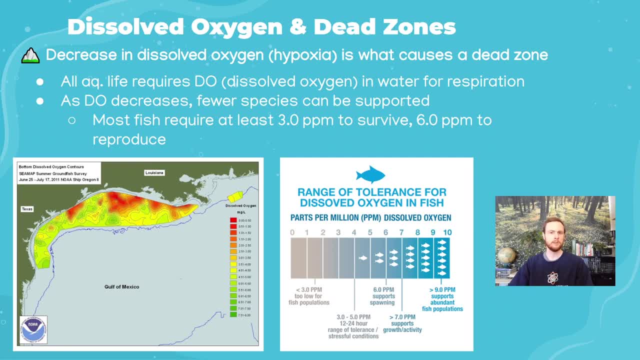 the five and a half parts per million range. So very little of the coastline of the Gulf of Mexico in the summer of 2011 could actually support a stable fish population, And so this is really important to help us understand the extent of eutrophication and the extent of the dead zones. 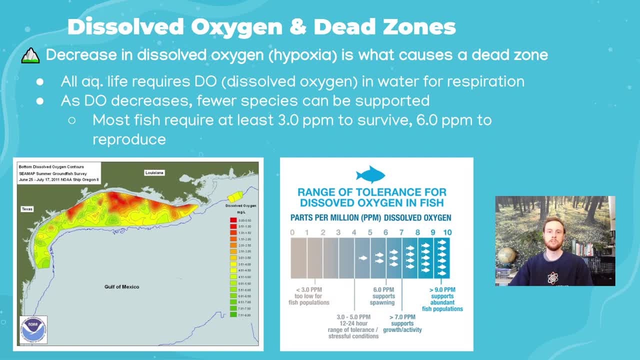 that can occur in the Gulf of Mexico as a result of all of the human activities that take place that dump a lot of these nutrients into the Mississippi River. And so it's again just a great kind of case study of how the Gulf of Mexico acts, kind of as a huge basin for all. 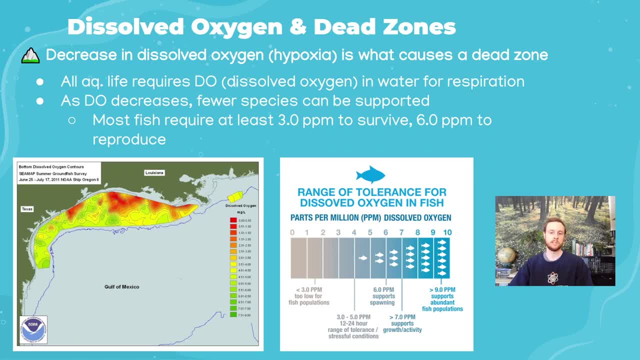 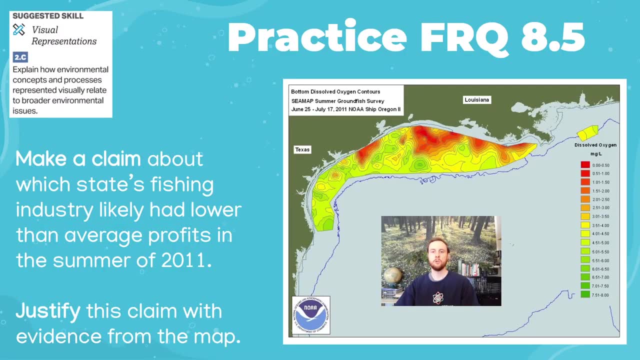 the pollutants from the land used really all over the Midwest and all over the South, And so we can see here the impact that that has on fish populations. So for practice, FRQ 8.5. I want you to take a closer look at this graph that we've just examined and make a claim about.